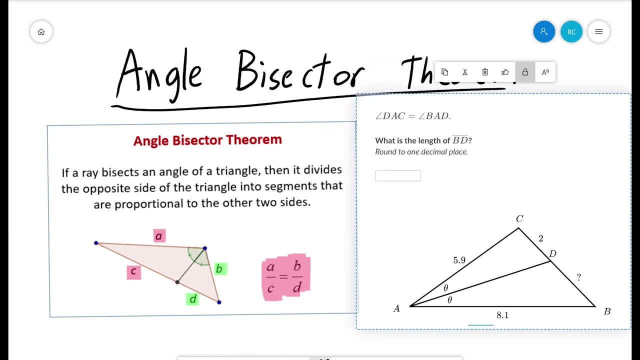 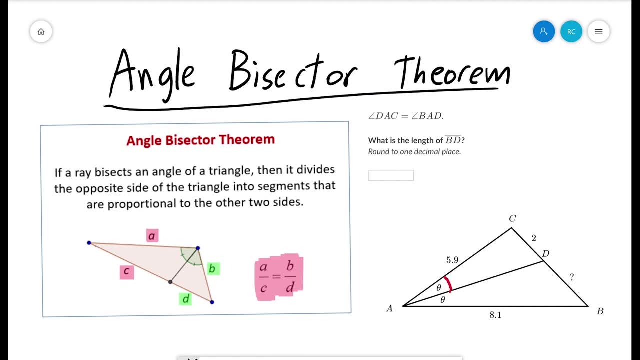 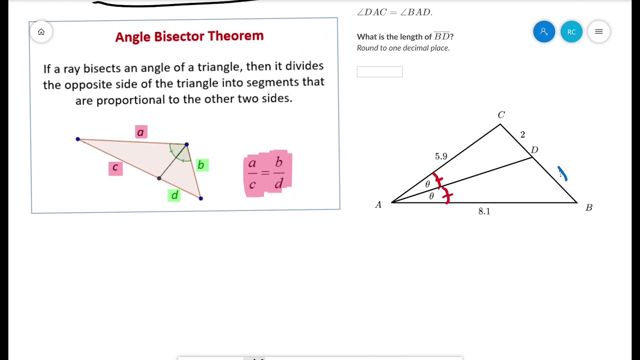 go. Okay. so it says that angle DAC- that's this angle right here- is congruent to angle bad- that's this angle right here. so those are congruent, which means we've got the angle bisector theorem. So what does the theorem say to do? Well, we're looking for it keeps. 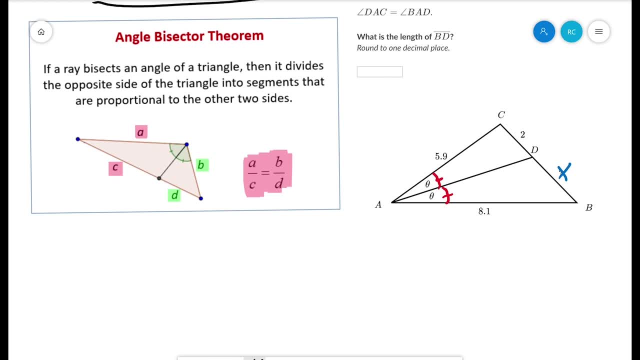 using a question mark. we're going to put an x there. we're looking for x. the bisector theorem says that in these two triangles the proportions of their sides are going to be equal, just like with similar triangles. So we can really jump directly to the end. 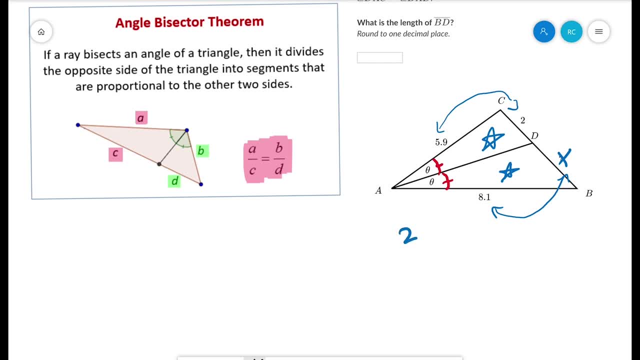 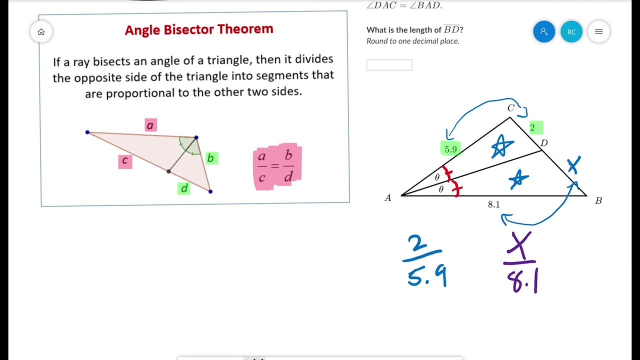 and say that 2 over 5.9, that's 2 over 5.9, and x- x over 8.1,. as you can see, I did the small side over the big side And those two proportions should be equal. 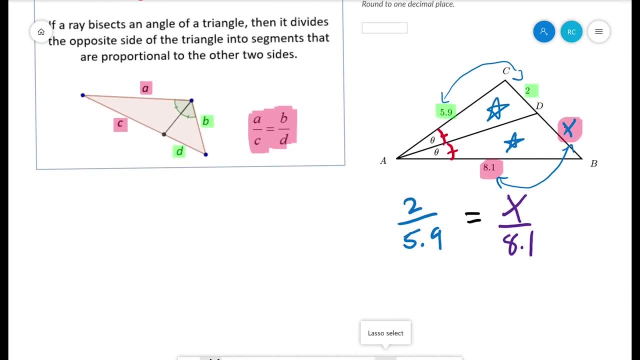 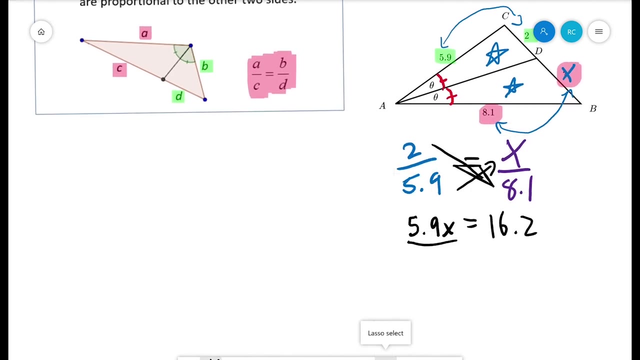 And now we're back to cross-multiplying. 5.9 times x is 5.9. x 2 times 8.1 is 16.2.. Divide both sides by 5.9.. Grabbing my calculator: 16.2.. 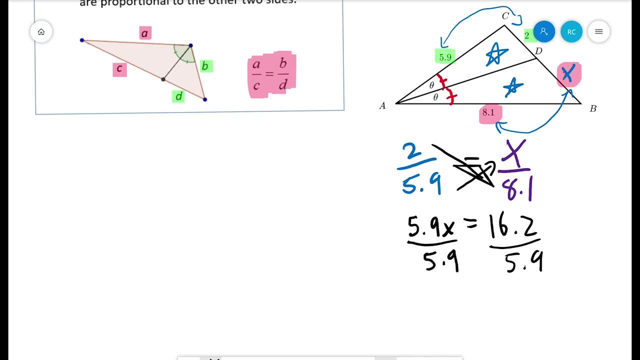 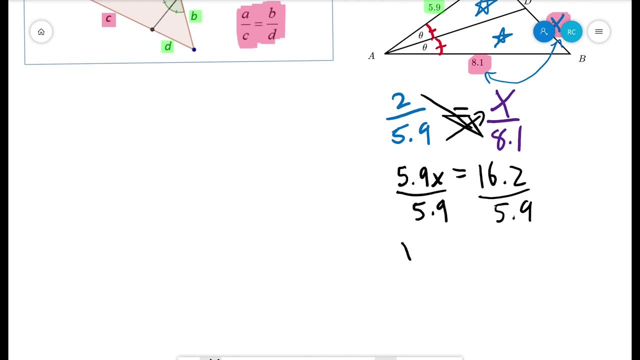 5.2 divided by 5.9 is 2.745.. Now it says to round to one decimal place. so we're going to say that x equals 2.74576, but since we're rounding to one decimal place, we're going to say that x is approximately. 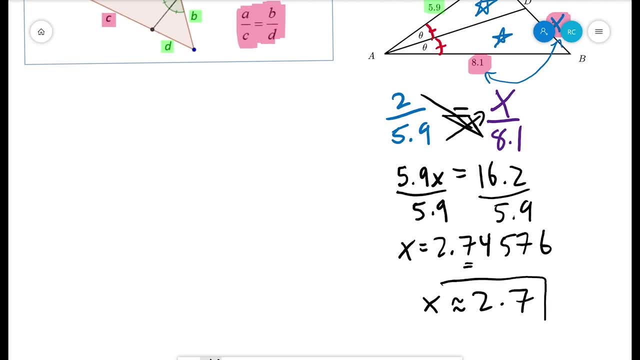 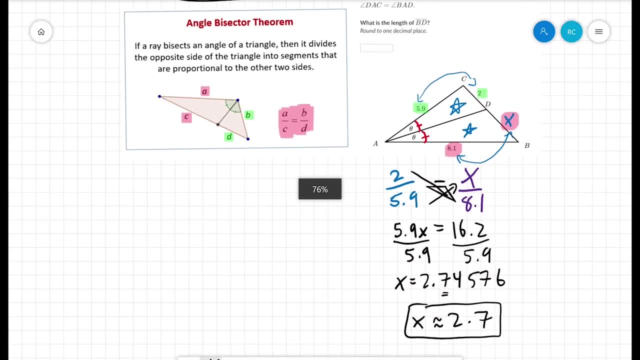 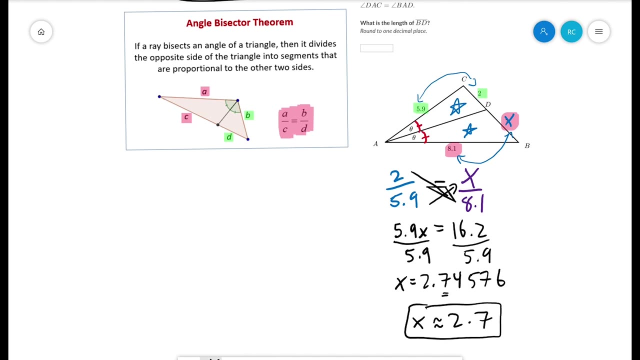 equal to 2.7.. All right, So again, it's just another proportion setup problem. The main reason I assigned this is not because the angle bisector theorem is going to be super, super important, but because I want you to get practice solving these proportions. 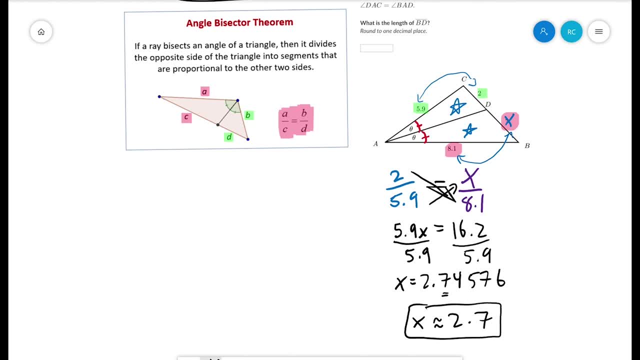 So we're going to copy one more of these. So we said x is 2.7.. Very nice. So here was example 2.7.. Very nice, Very nice. Here's example 1.. Here's example 2.. 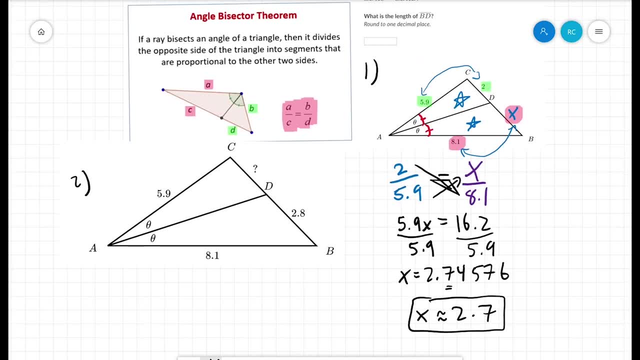 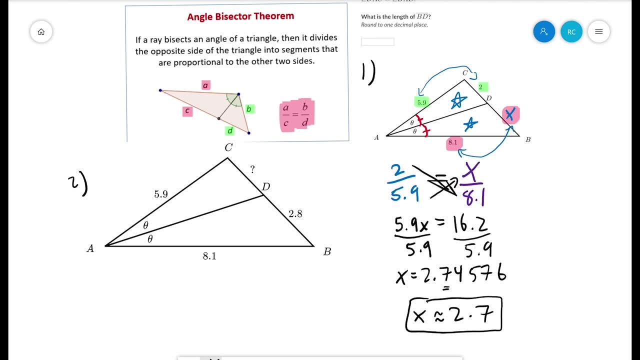 OK, So again, go ahead and pause the video for a moment and see what you can do with this on your own, please. This is our first day of class, so I am trying to start things off kind of slow, but I do. 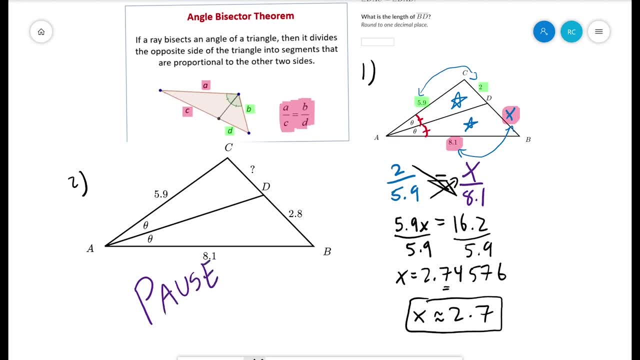 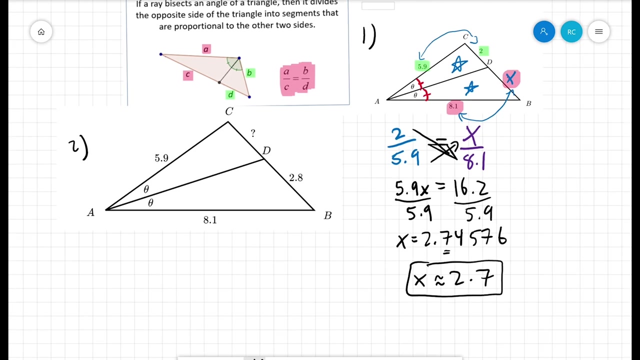 want you to go ahead and hit that pause button. grab a piece of paper, see if you can solve for the question mark which is side CD Ready set. go Now. I'm sure you all went ahead and paused the video and did the thing. I'm sure. 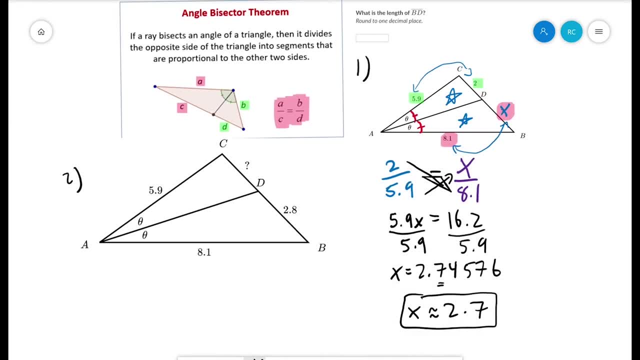 So here's what we're going to do. We're going to do the same exact thing By the angle bisector theorem. we can say that, for example, x over 5.9.. That's x over 5.9.. 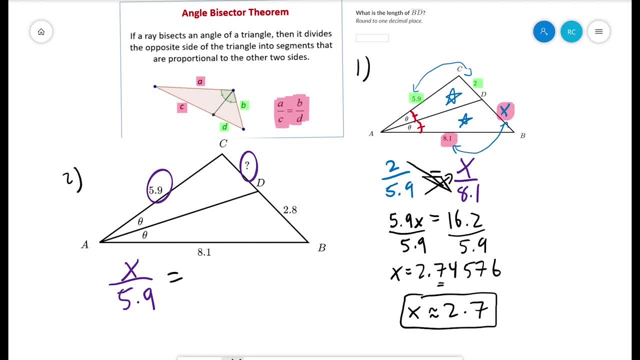 Equals 5.9.. Equals 2.8 over 8.1.. So again, we went this way, but we could have gone the other way. You could have done 5.9 over x and 2.8 over, or 8.1 over 2.8.. 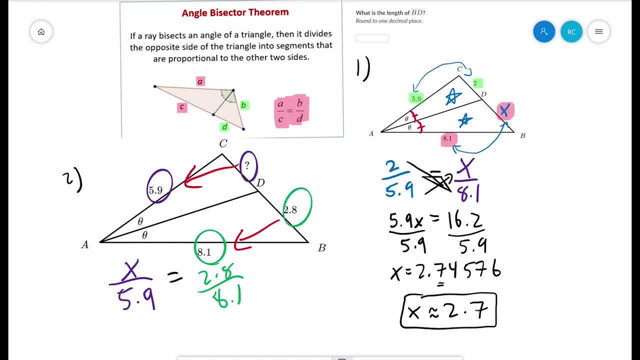 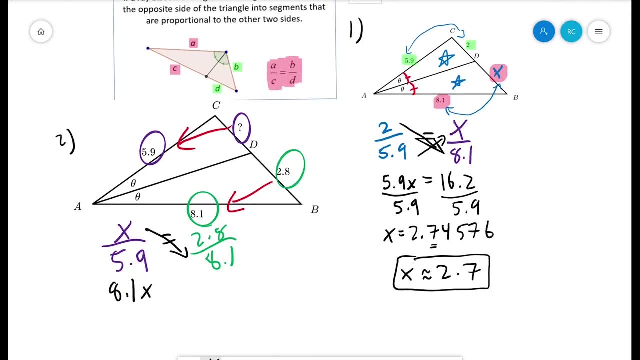 That would have worked just as well. Now we're back to cross multiplying. Let's see: 8.1x equals, uh, 5.9 times 2.8,. let's see: 5.9 times 2.8 is 16.52,. divide both sides. 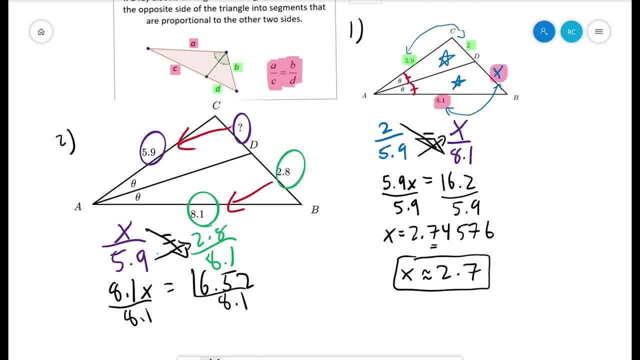 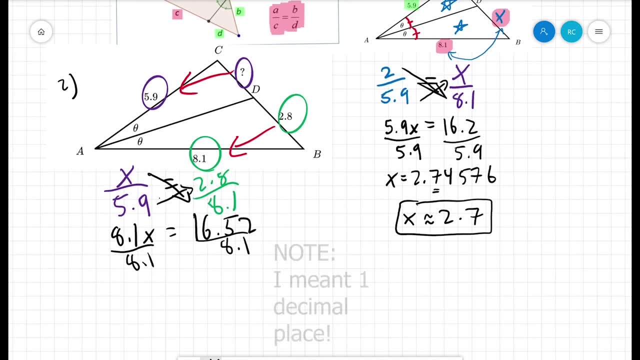 by 8.1, we're going to get a little bit more than 2.. Divided by 8.1, we get 2.039.. Now again we're rounding to two decimal points. So we're going to say x is a product.